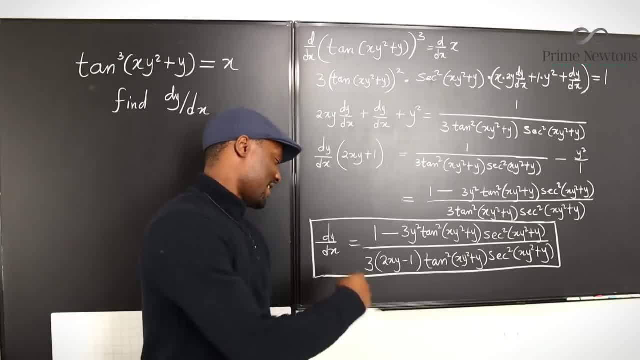 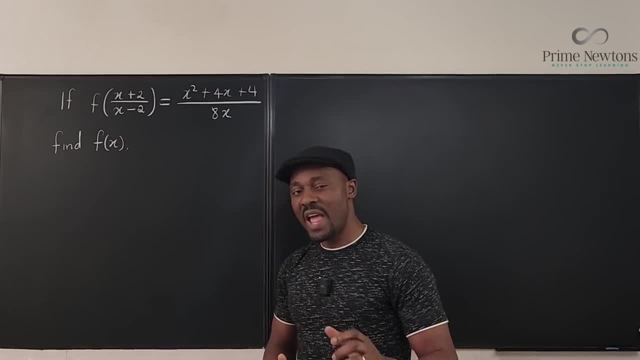 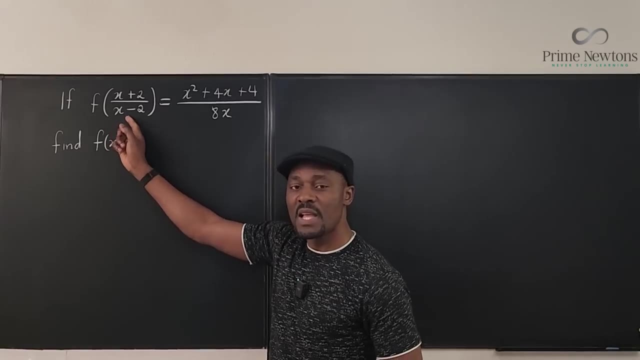 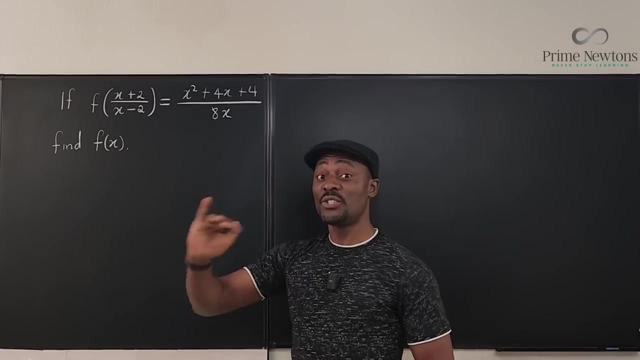 Here is my suggestion: Whenever you get a functional equation- if it is just one single function that is involved in it, like this one, try to plug in a very convenient number and see what you get on the right hand side, so that when you get your final answer, you 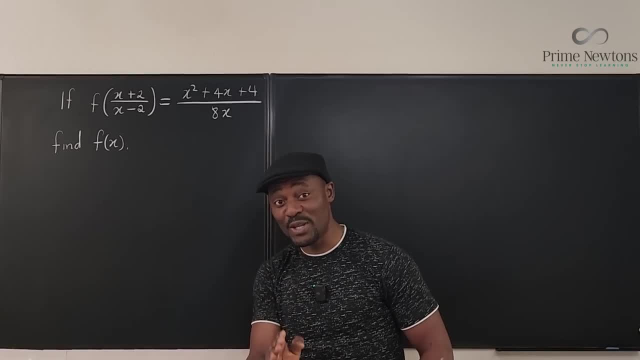 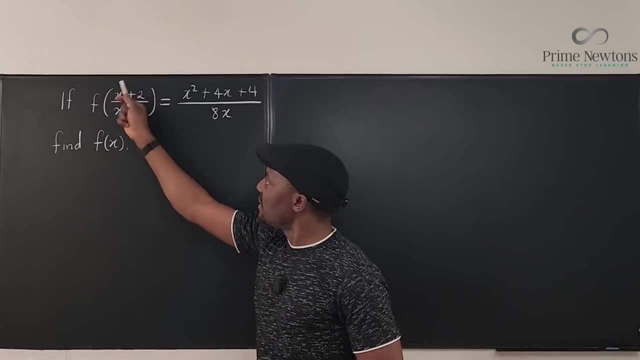 can test it and see how it works. So this is what I usually do. I would say I want to make this equal to zero. Okay, So when this is zero, I want to know what's going to happen on this side, because when I get my answer, it's easy to. 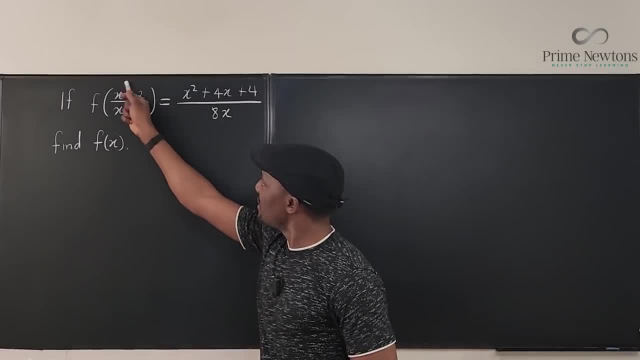 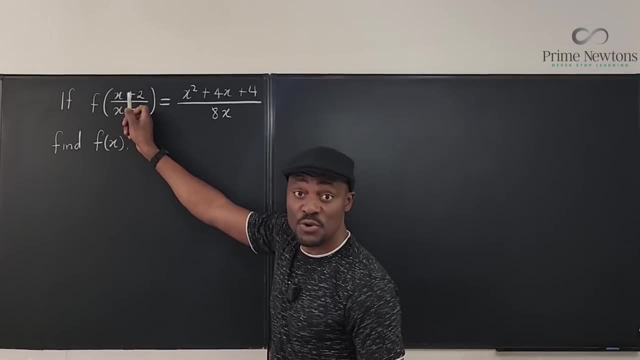 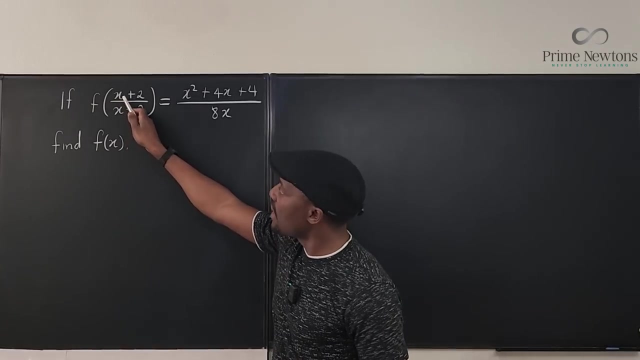 plug in zero. Okay. So if I want to make this argument zero, what I'm going to do is: I know the denominator can't be zero, but I can make the numerator equal to zero by making X to be negative two. So if I assume that X is negative two, it's going to be negative. 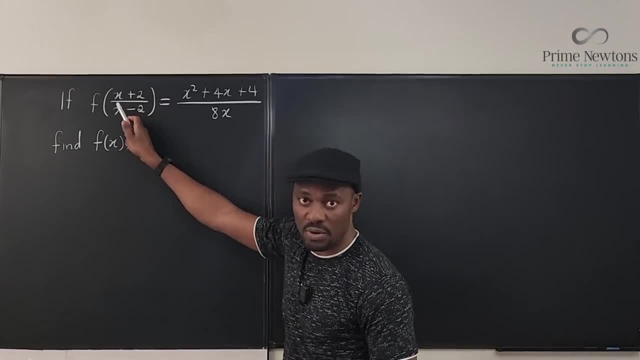 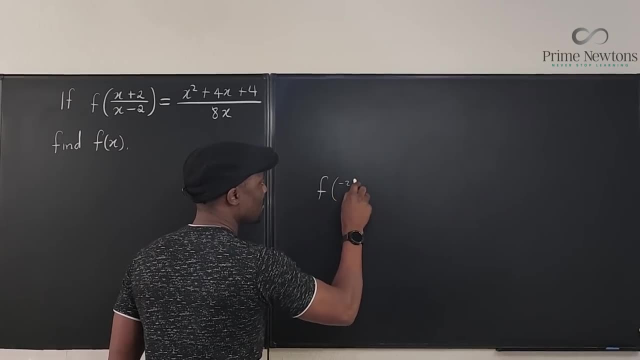 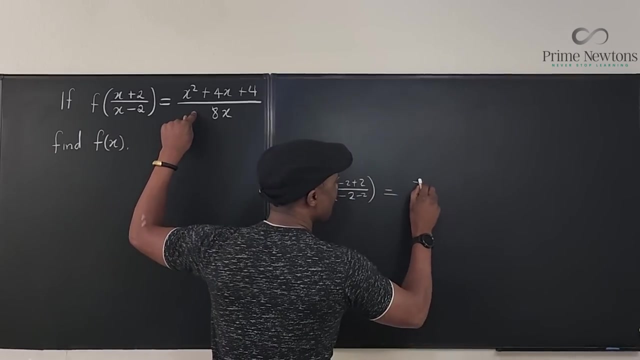 two plus two, which gives me zero over negative four. So this is F of zero. So I'm going to be having watch this. it's going to be F of negative two plus two over negative two minus two, And here it's going to be negative two squared plus four times negative two plus 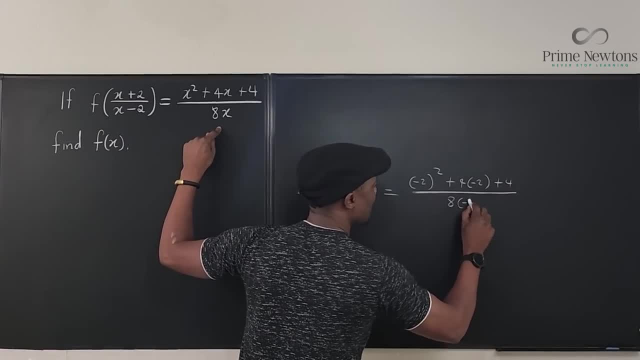 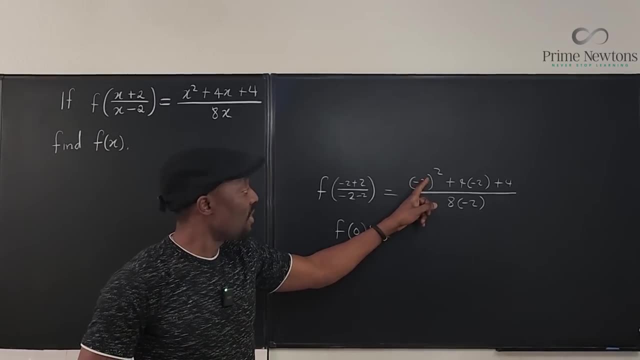 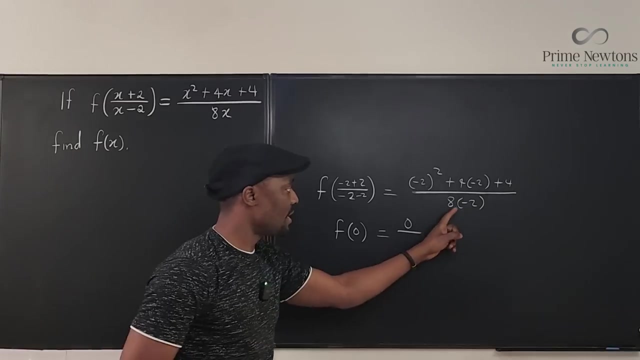 four divided by eight times negative two- Here I know I have F of zero And here I'm going to evaluate- I'm going to get four minus eight plus four, That gives me zero. on top And down here it's negative 16.. So equals zero. So I know that by the 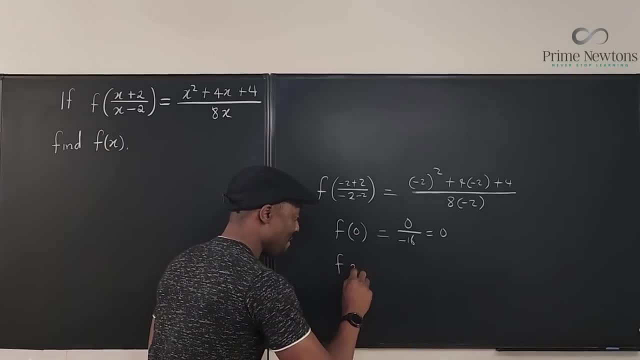 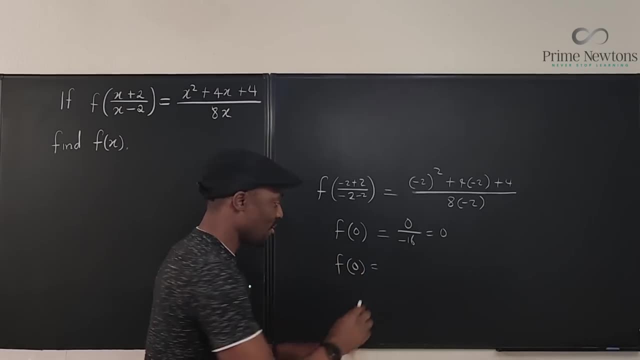 time I get my final answer, I'm going to have. F of X is equal to something, But when I plug in zero in that function, I'm going to get zero. That's a quick test for me to know that. Okay, This function I just claimed I got may be true. Now, just to be sure you should try. 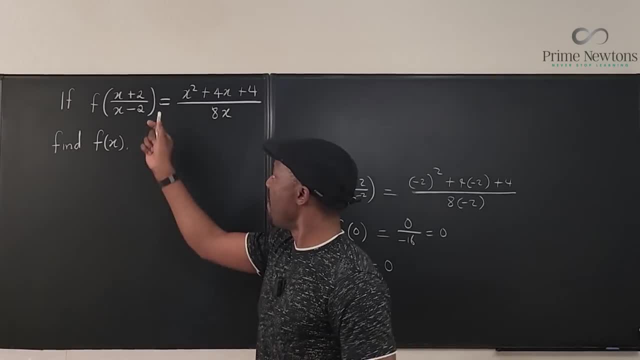 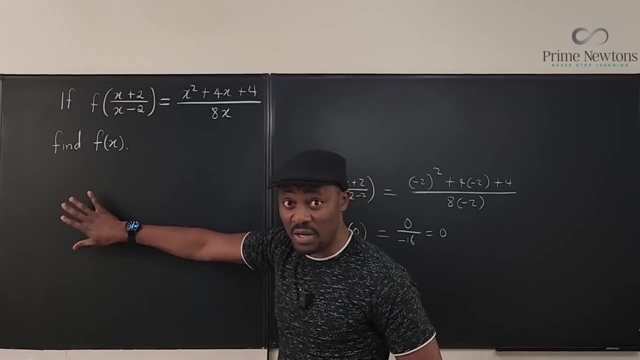 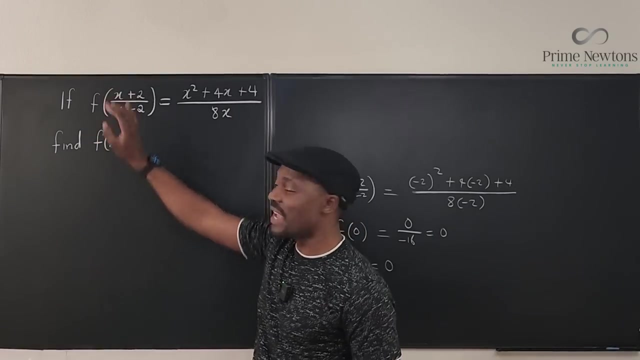 two or three different values to make the argument of this before you start. Okay, So how do you start? This is a very easy one, because you only have a single function. In the more complicated ones, you're going to have F of this and you have another F defined. 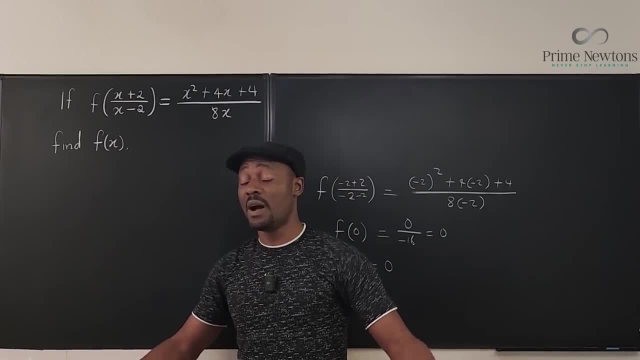 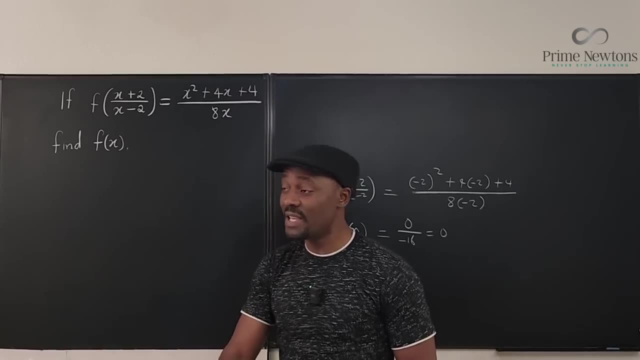 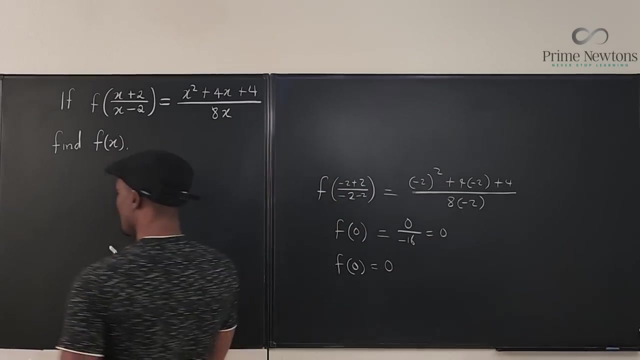 in another way. So the number of steps you're going to take will be multiple, But this is a very easy step. And what should you do? The only thing I would recommend is replace everything in here with another letter. That is the strategy. So we're going to say: let 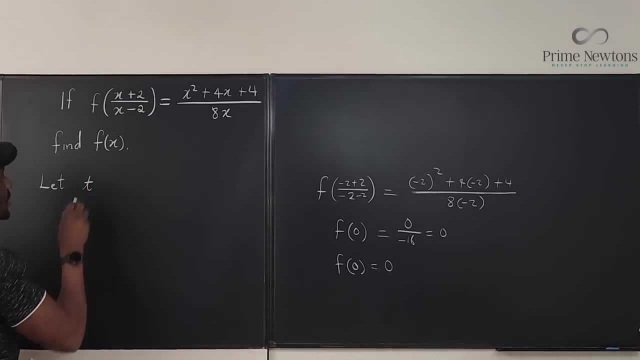 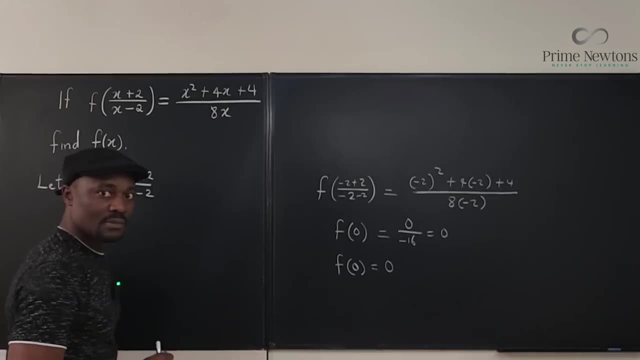 T. I like using T be equal to X plus two over X minus two. Okay, So that when I write this function next I'm going to say F of T And that's it, That's it, That's it, That's. 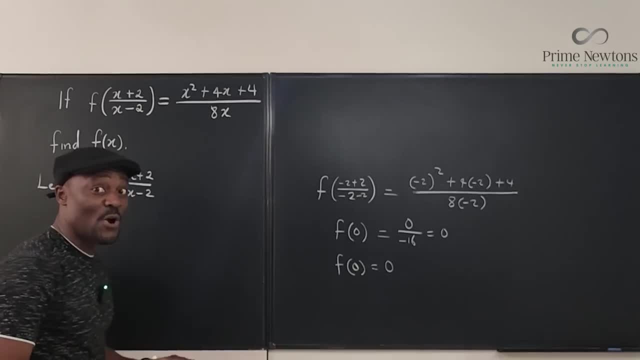 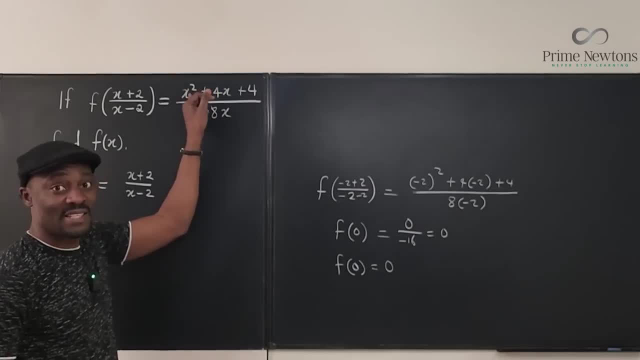 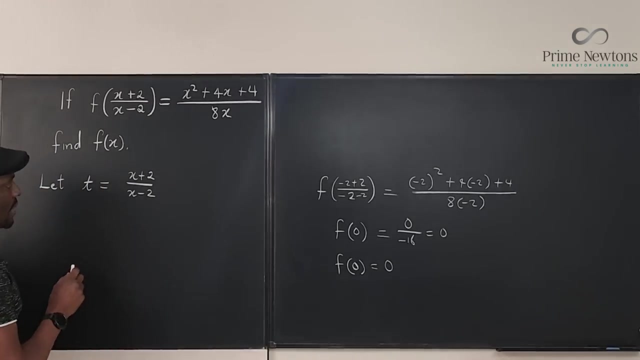 crazy. Why? Because we have to replace X with T. Okay, So if we say T equals X plus two over X minus two, Well, we need to isolate X so we can go replace it with something in terms of T. So let's clean this up. So we're going to have T times X minus two will be equal to. 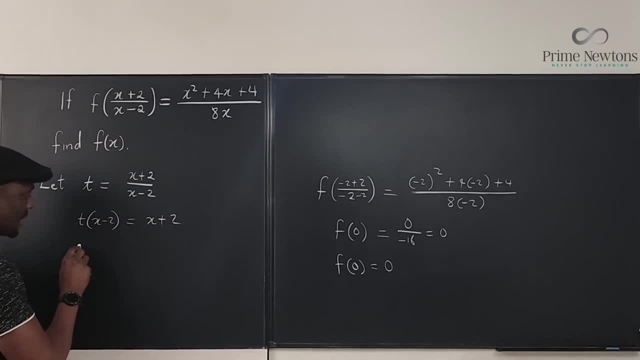 X plus two, And then we have Xt minus. 2t equals X plus 2. put all the X's together, we got Xt minus X will be equal to 2t plus 2, so that X will be equal to, let's, factor X. we have T minus. 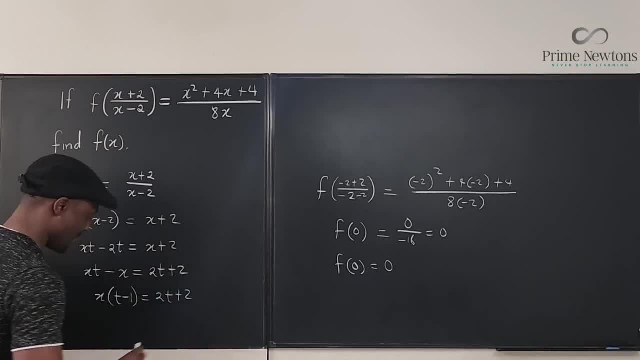 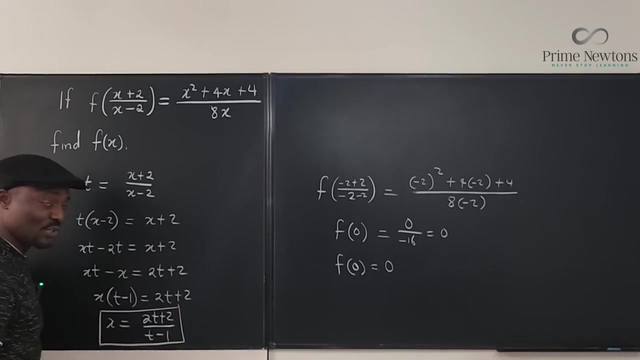 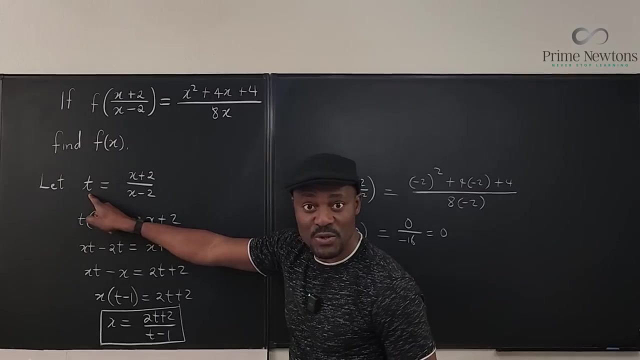 1 equals 2t plus 2, and what do we have left? we've got X will now be equal to 2t plus 2 over T minus 1. this is the key to where we're going. once you've been able to replace X with this letter T that we use a substitute, now we're gonna. 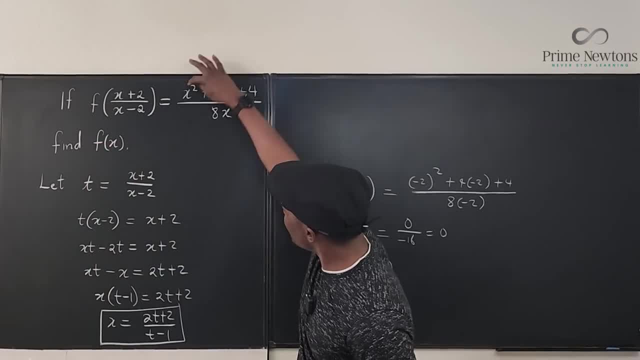 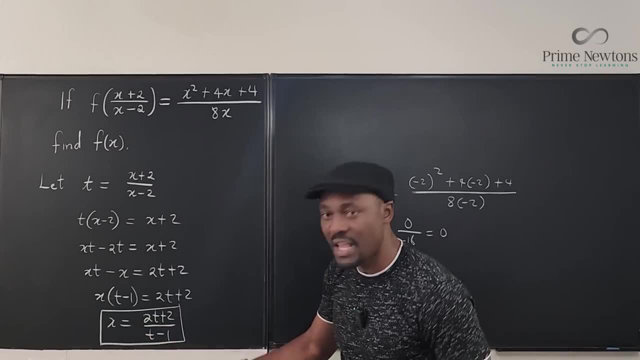 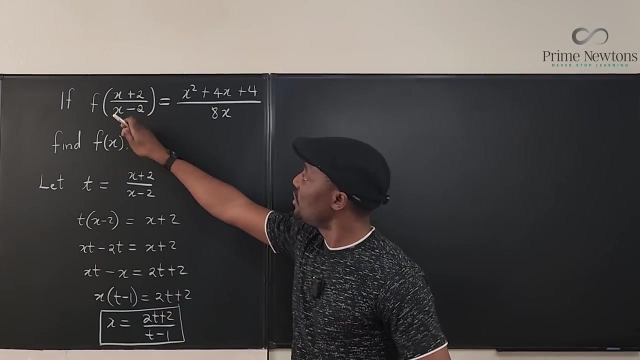 say, f of T will be equal to- instead of writing x, squared plus 4x plus 4 over 8x. everywhere you see X. you're going to replace it with this. you simplify and you get your function. so let's go back to what we have to do. this is now f. 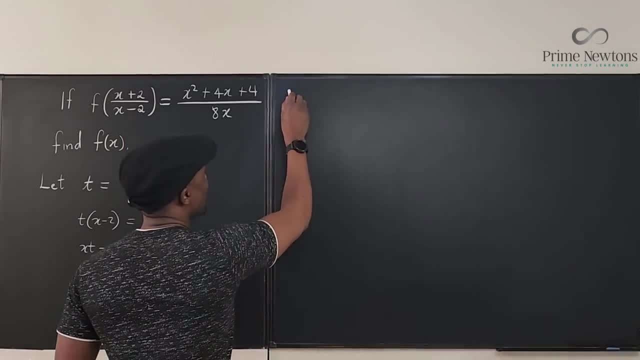 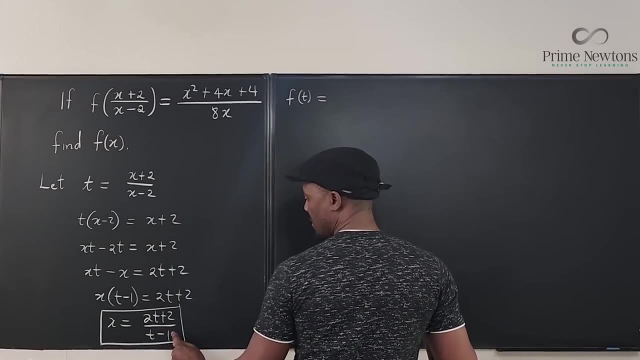 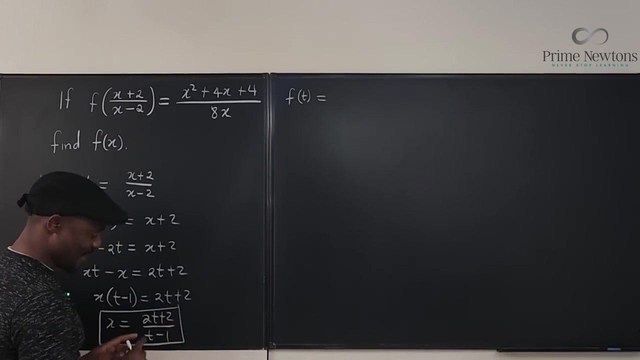 of T. so we're gonna say f of T is equal to x squared, but we said X is this now, so I'm going to write this, I'm gonna square this. okay, this looks like 2t, T, 2. no boys, 2t plus 2, okay, so I'm going to factor out the 2 and just write this. 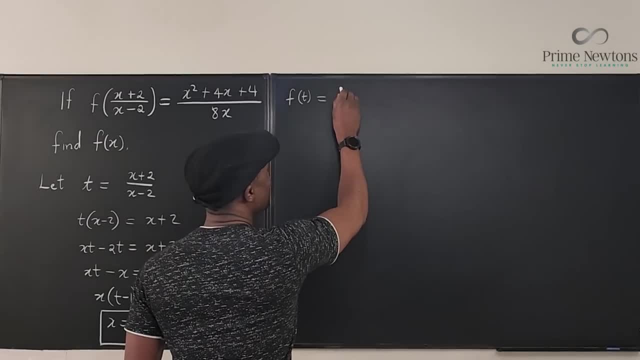 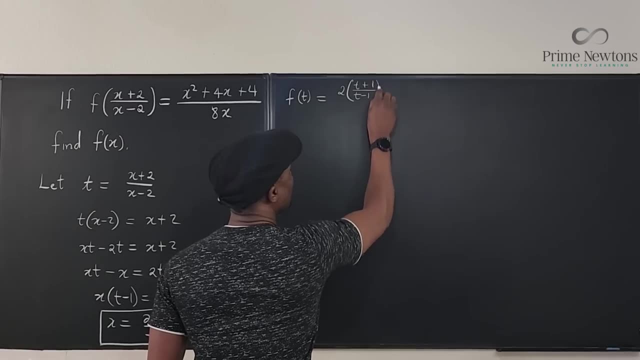 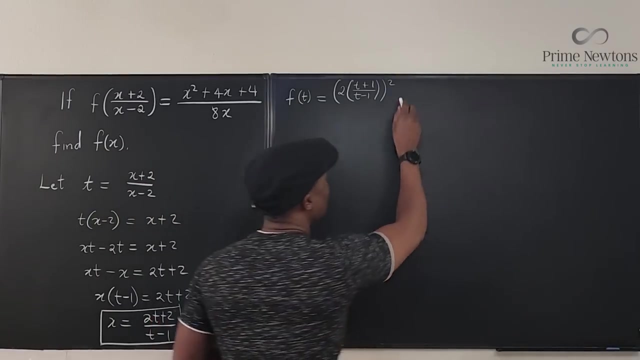 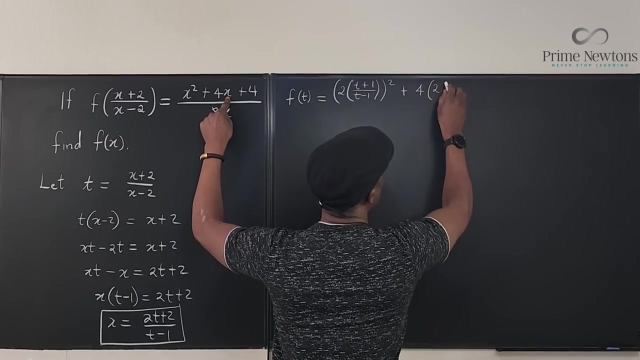 as T plus 1 over T minus 1. so this is going to be 2 times T plus 1 over T minus 1. everything squared, that is x squared. I'm going to go to the next one and say plus, this is going to be 4x. that's going to be 4 times 2 times X plus. 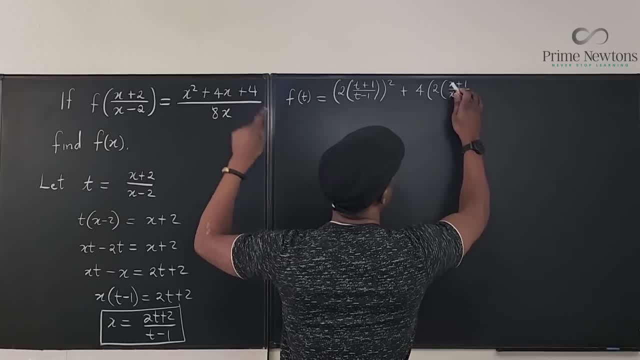 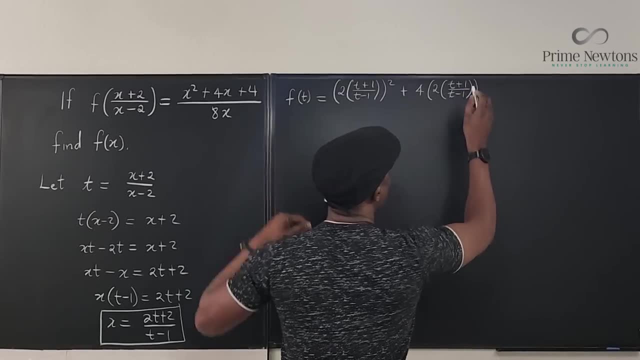 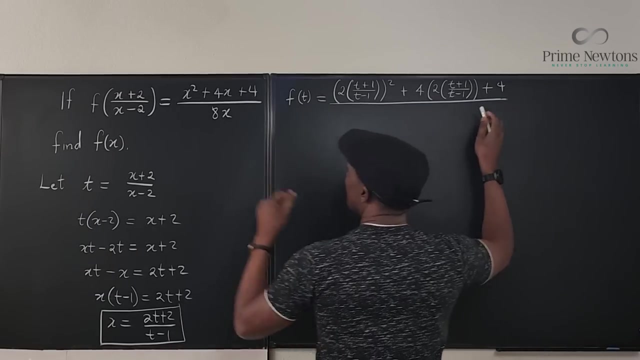 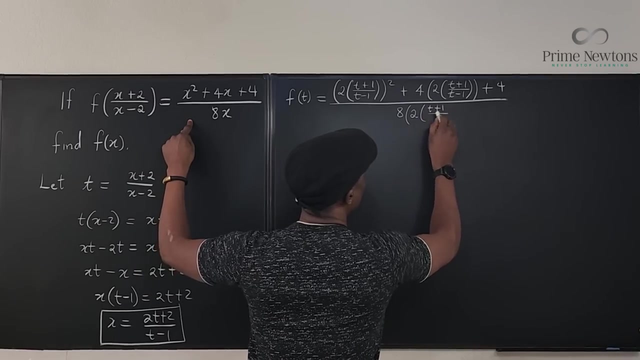 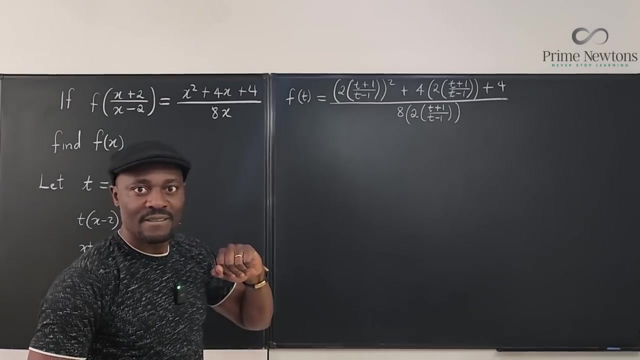 1 over X minus 1. sorry, not X T. T plus 1 over T minus 1. okay, and plus 4, all divided by 8 times 2 times T plus 1 over T minus 1- okay. so what do we get here? nothing special. 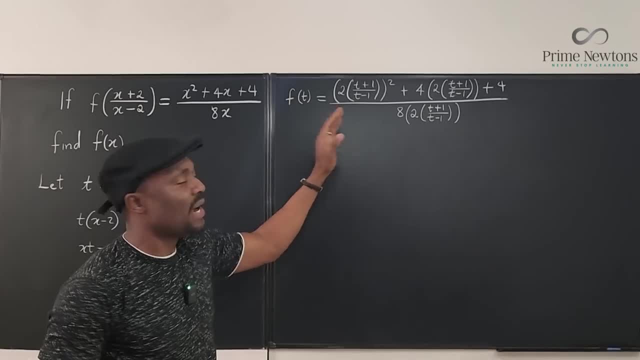 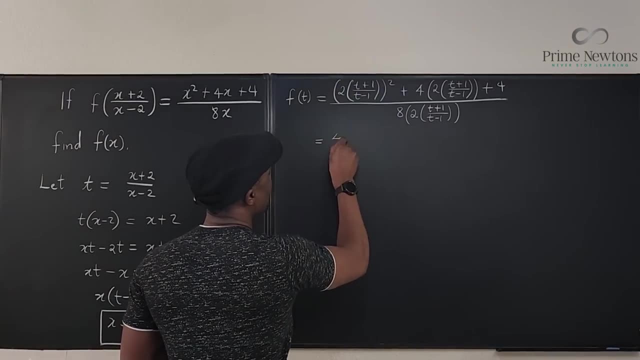 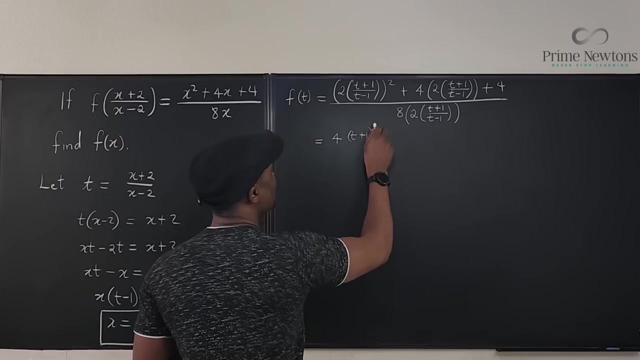 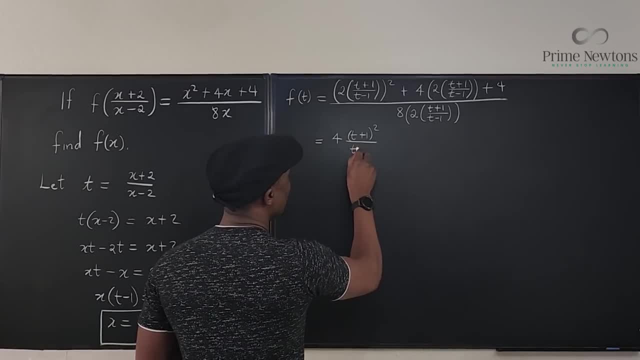 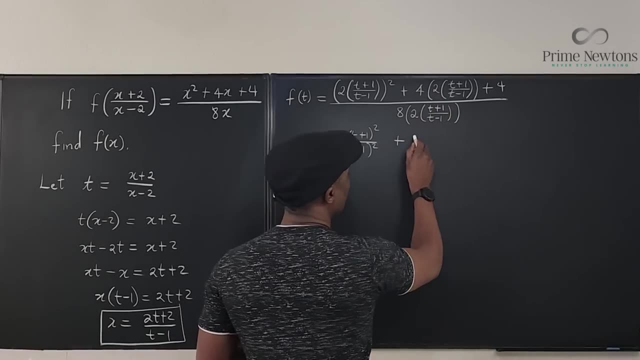 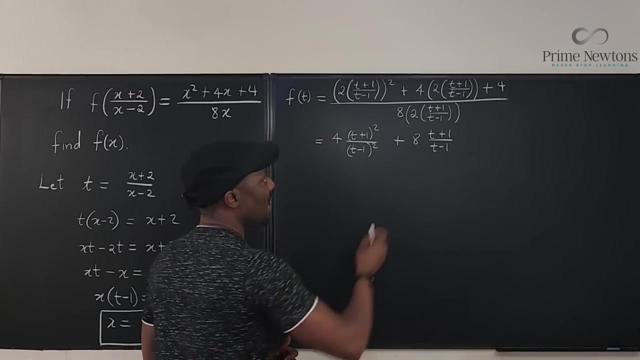 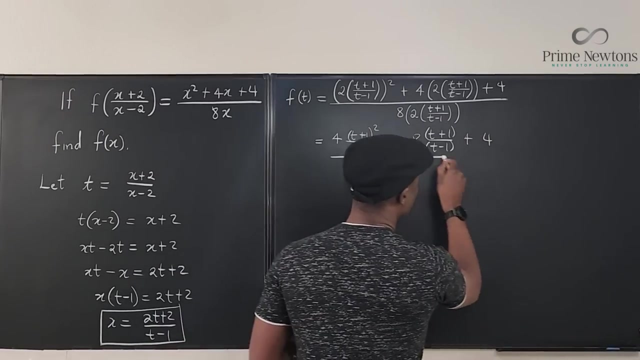 squared over T minus 1, squared nice. plus 4 times 2 is 8. so I'm going to write 8 here and write T plus 1 over T minus 1. okay, I'm going to put it, let's just do it this way: plus 4 and everything here is divided by 16 times. 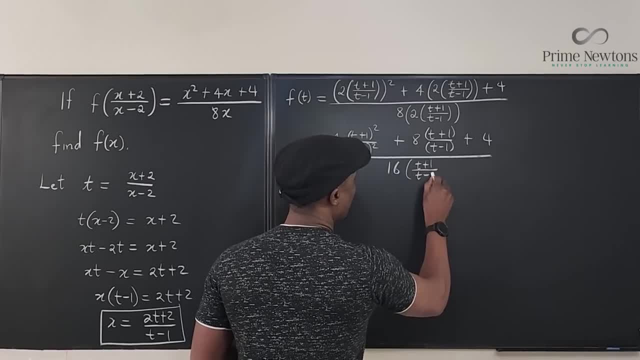 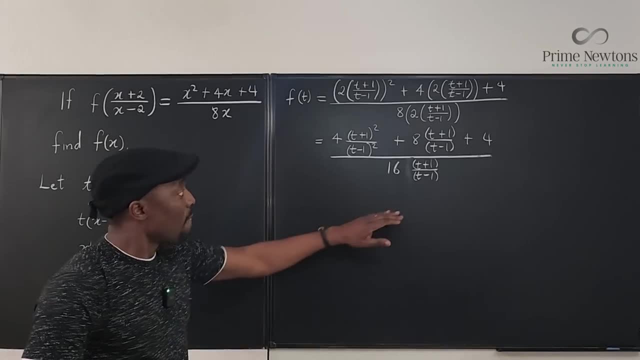 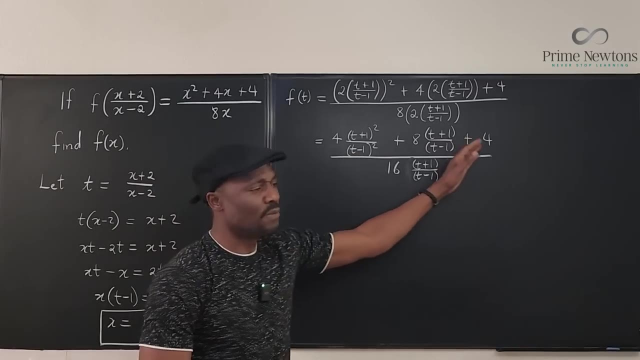 T plus 1 over T minus 1, let's separate them. okay, let's do it this way, just leave it that way. now we're almost there done. If only we can just look at what we have and say: hey, I have too many fours, or I have 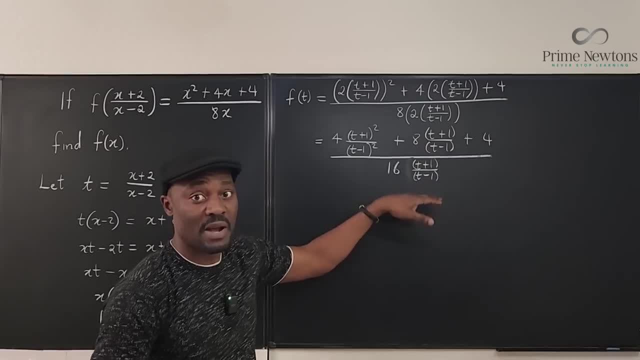 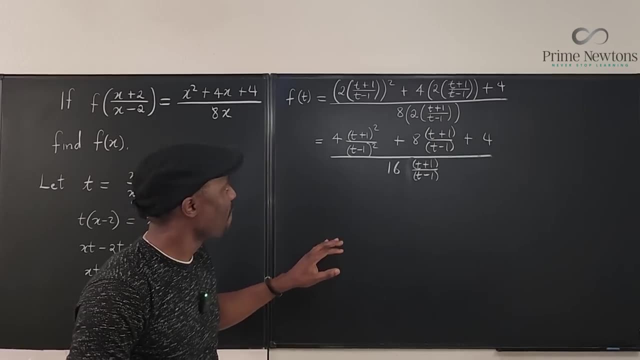 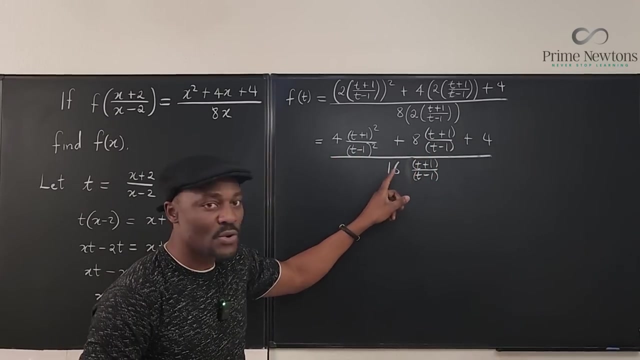 fours everywhere. So divide the top and bottom by four. That's one step. I want to do many things at the same time because I want us to get to our answer Now also. look at all. This is a complex fraction. Look at all the denominators that you have. You got t minus one is a denominator. 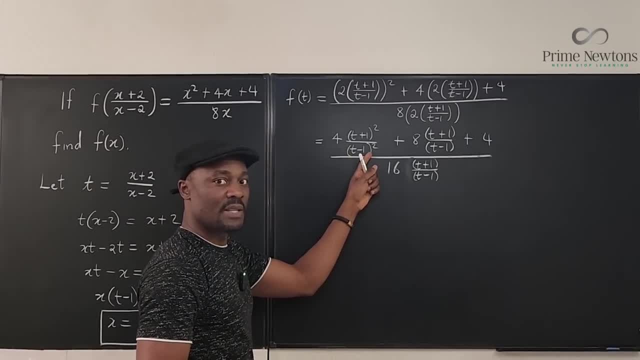 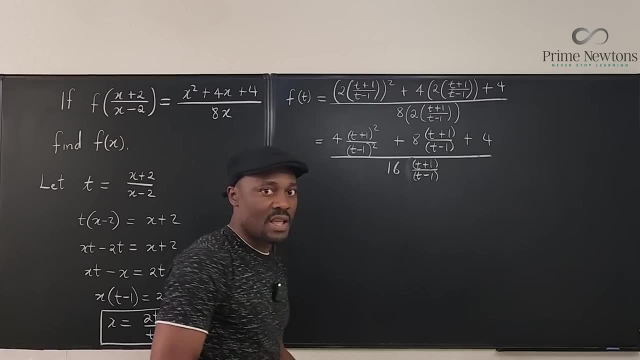 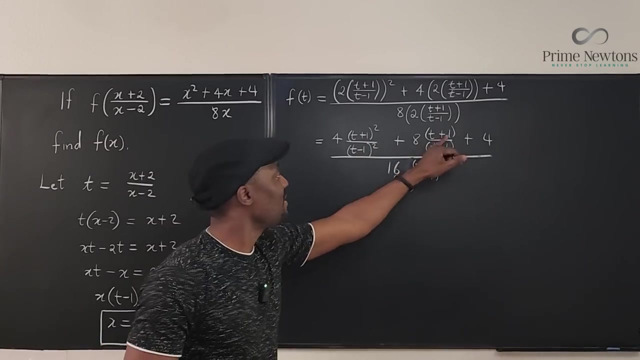 here: T minus one squared is a denominator. here. T minus one is a denominator here. So if we pick the highest denominator on top and on the bottom, everything looks like: yeah, t minus one squared is what we should use. I'm going to be multiplying everything by t minus one squared and I will be. 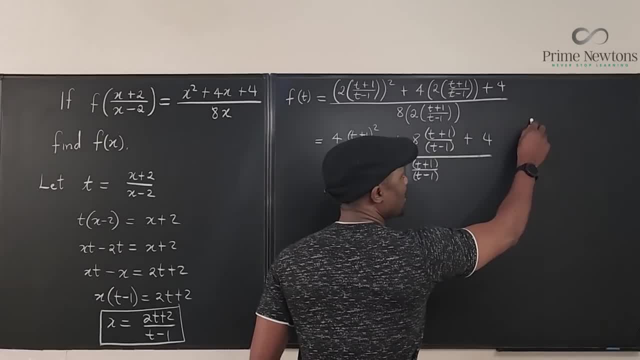 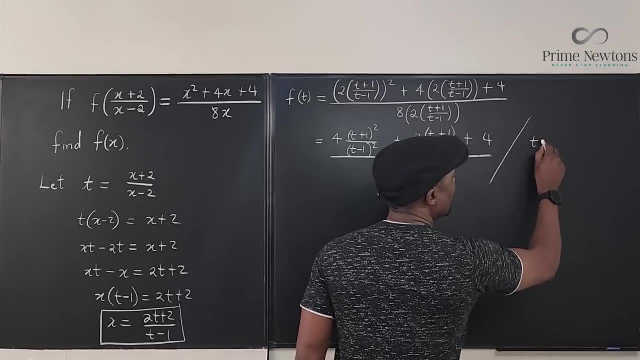 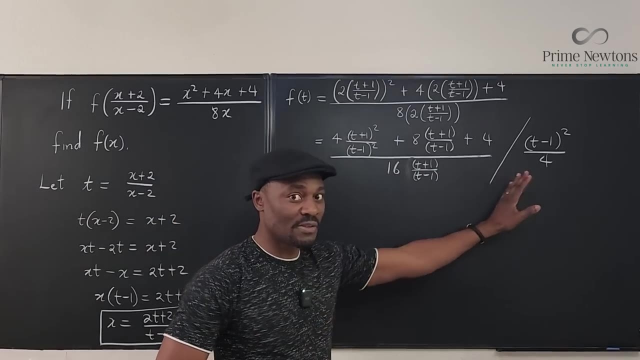 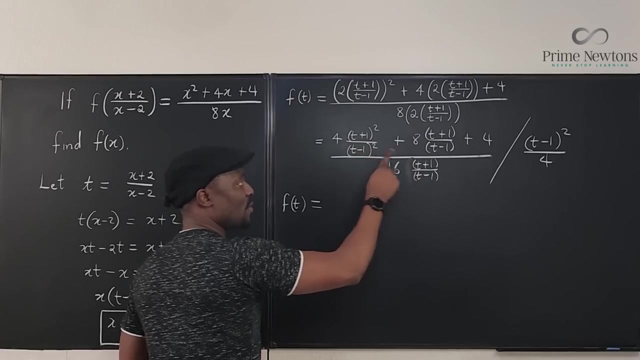 dividing everything by four. So this is what I'm going to do: I am going to multiply by t minus one squared. t minus one squared over four. That takes care of most of the things I'm worried about right now. So let's begin. If I use this to multiply this, this t minus one squared will cancel this out. 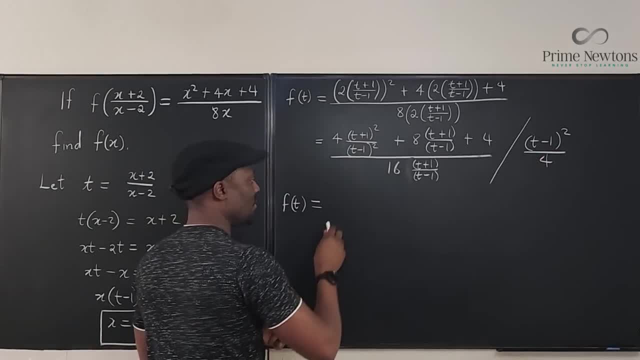 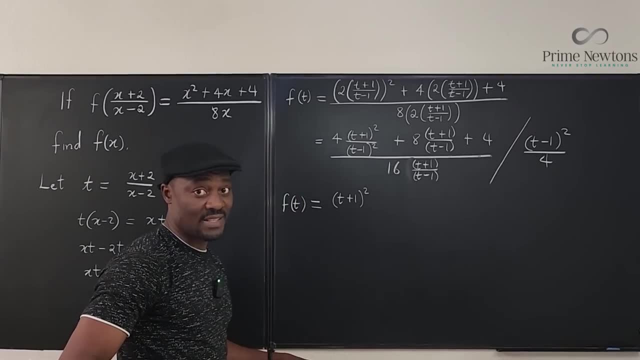 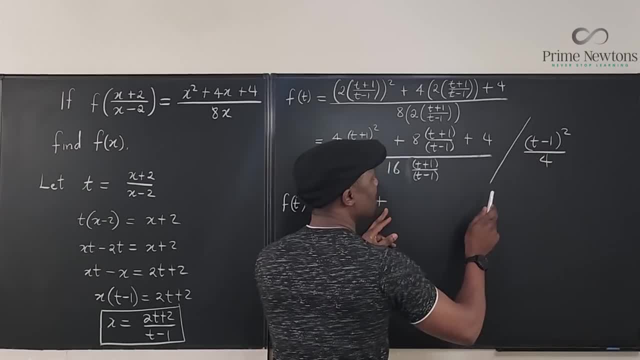 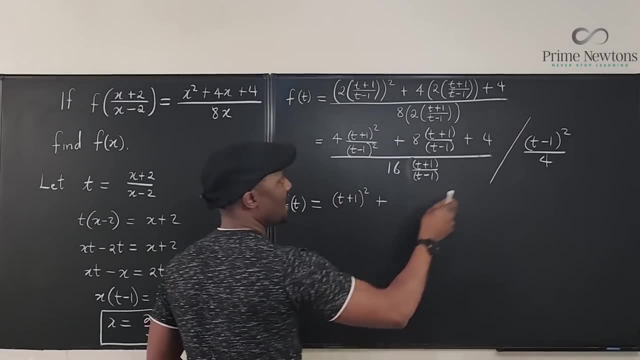 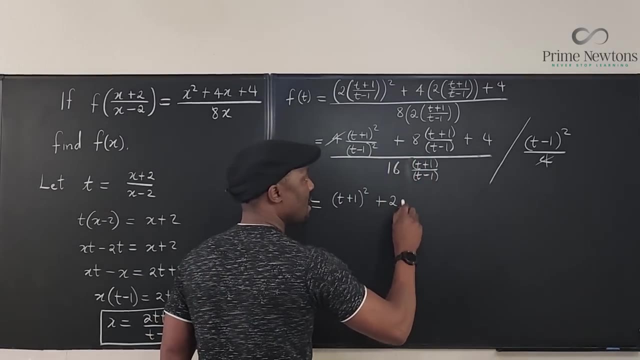 If I, this will cancel out one of these, What I have left will be t minus one. I use it to multiply this. It's going to give me: oh, the fours should go. actually, This four should take care of this four, This four should take care of this, And you have two. So I'm going to have two And then I'm. 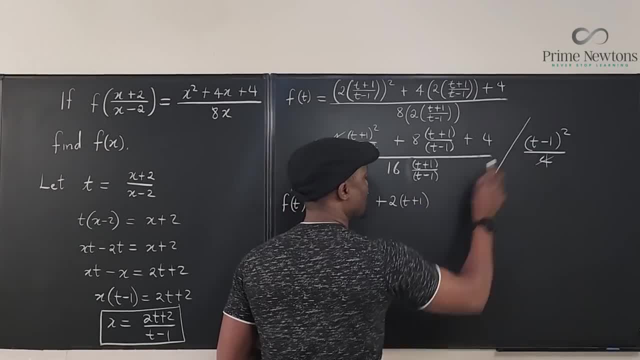 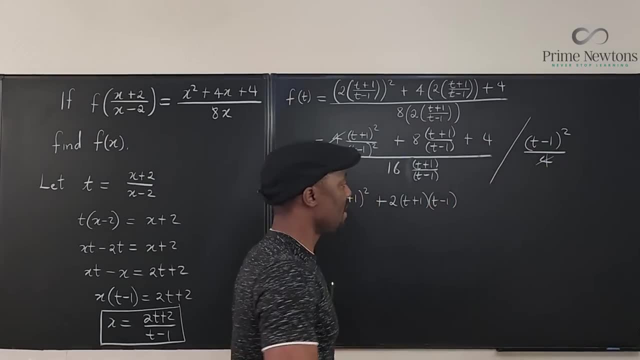 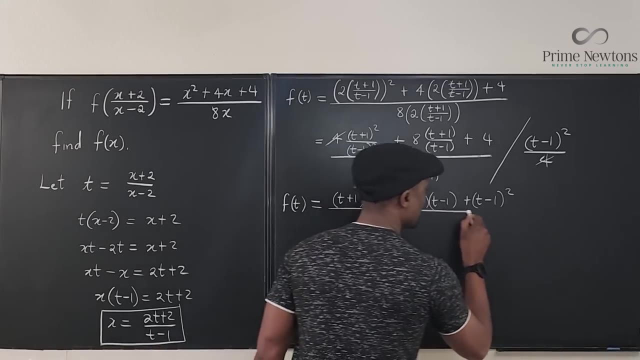 going to have t plus one times one of these, which is t minus one, And then this takes care of this, And I'm going to have t minus one squared plus t minus one squared, And all of these will be divided by. So this four is going to take care. 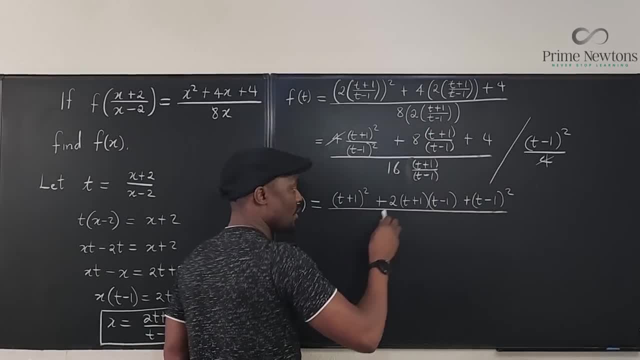 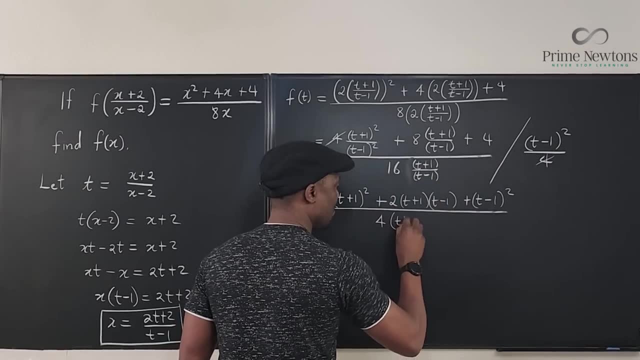 of this. Remember: this means I'm doing it to the top and the bottom, So I'm going to have four left here, And then this will take care of one of these. The other one is going to be t plus one, t minus. 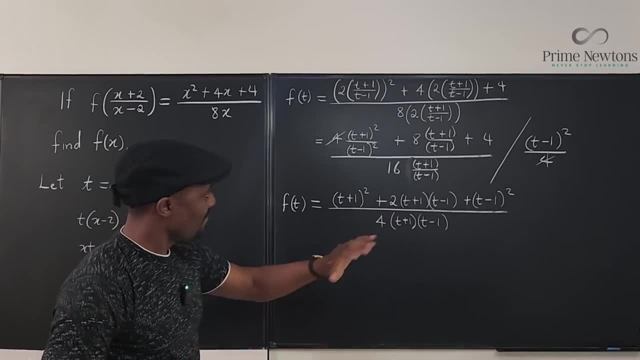 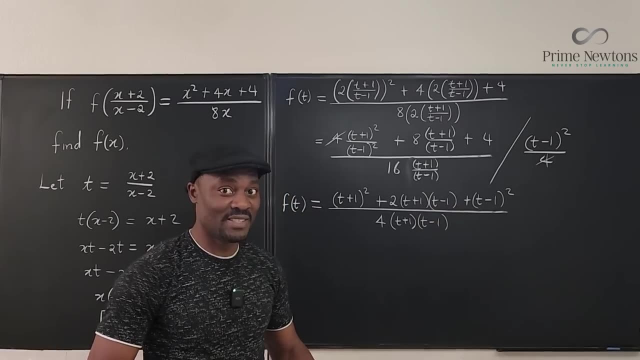 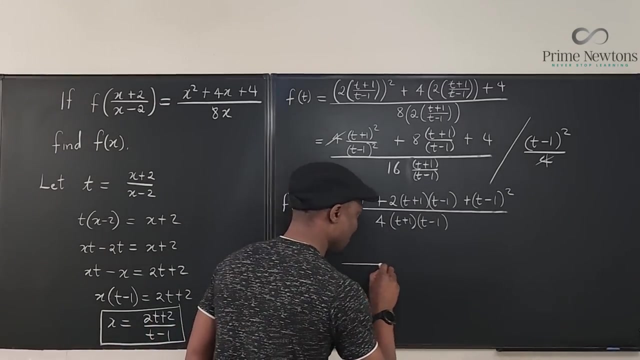 one, Okay, So we're almost there, because now I can rewrite everything. In fact, let me just do it. It's going to be crazy, Okay, But hey, this is difference of two squares, So let's just do this. So if I write this, what I have here is four times the difference of 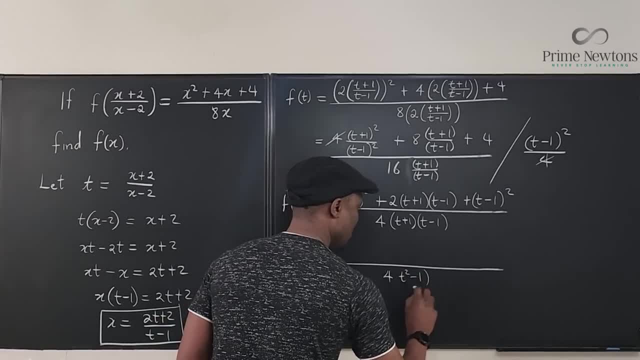 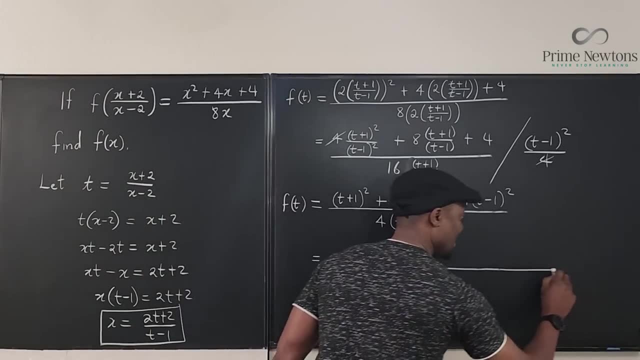 two squares, which is going to be t squared minus one. That's another way to rewrite this, But let's work on the top, because the top is the part that's insane. So if I distribute this, what do I get? I'm going to get: 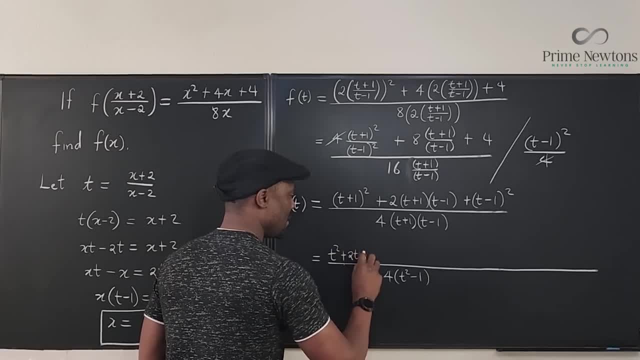 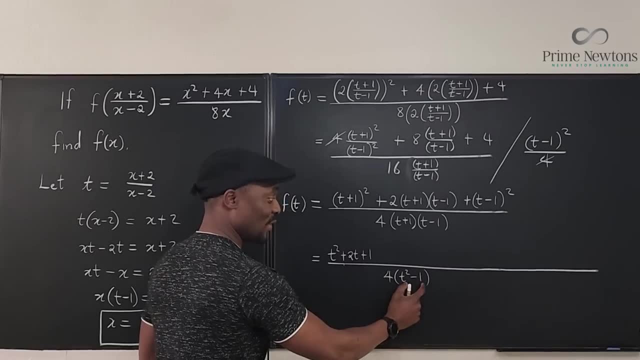 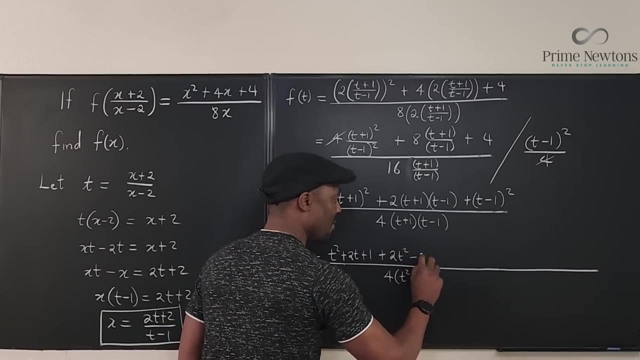 t squared plus two, t plus one. Go here: Oh, this is difference of two squares. It looks exactly like this, And I need to multiply it by two. So it's going to be plus two, t squared minus two. That's what this is going to give us, because it's this one multiplied by two. And if I go here, 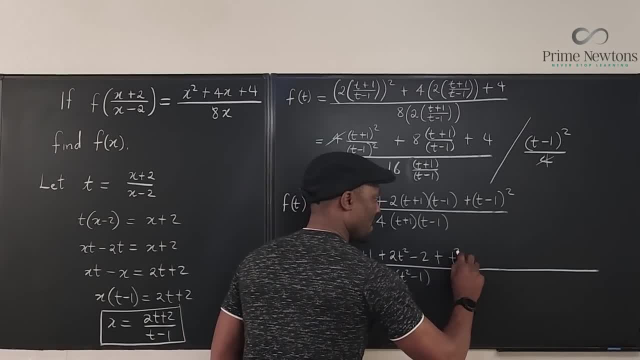 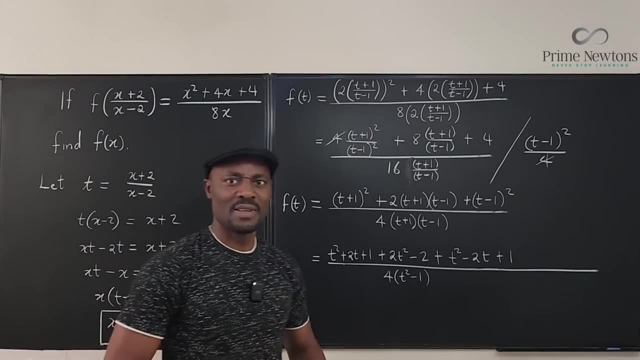 well, I'm going to do the same expansion. It's going to be two squared minus two, t plus one Plus one. It's not as bad as I was thinking. Come on, That was an exaggeration. Let me see if I can. 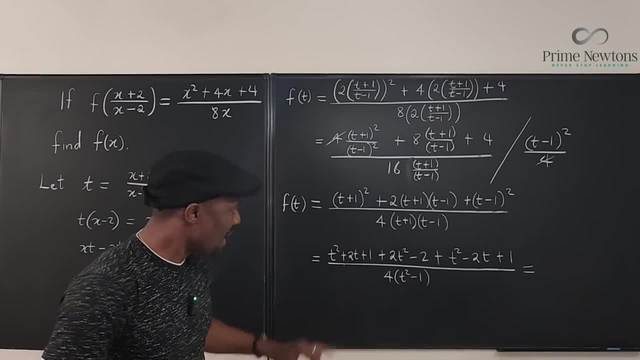 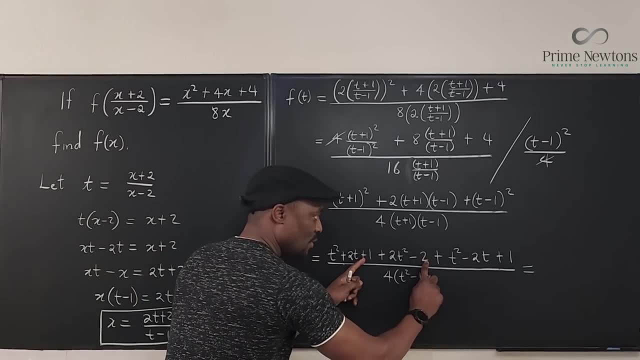 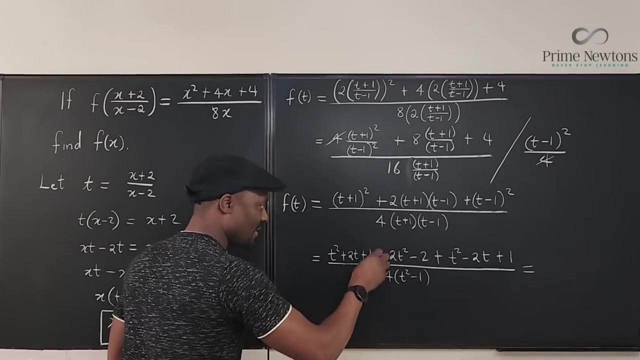 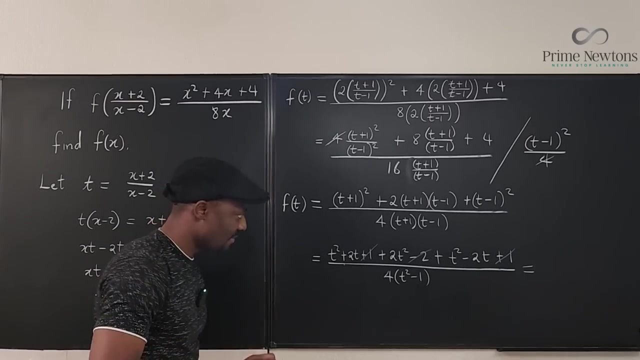 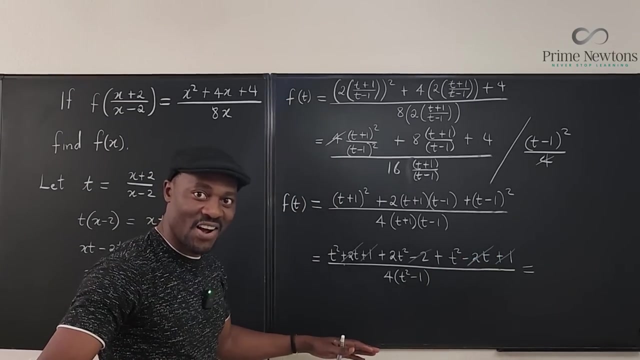 squeeze in something on that side. What can we do here? I know that one plus one minus two is zero. So all the numbers are gone. Right, One plus one minus two gives me zero. Now let's go. I know that two t minus two t is gone. Now I have t squared plus two, t squared plus t. 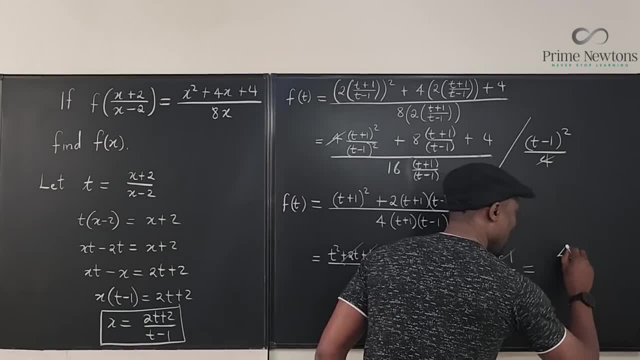 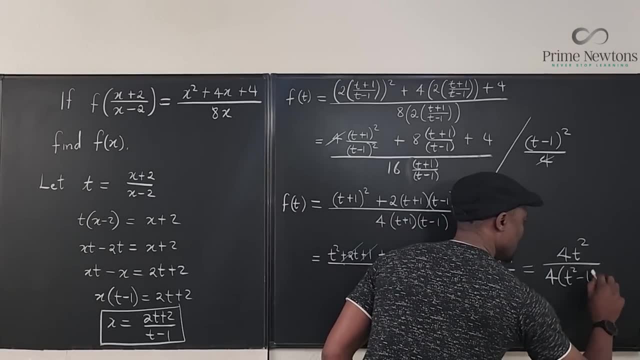 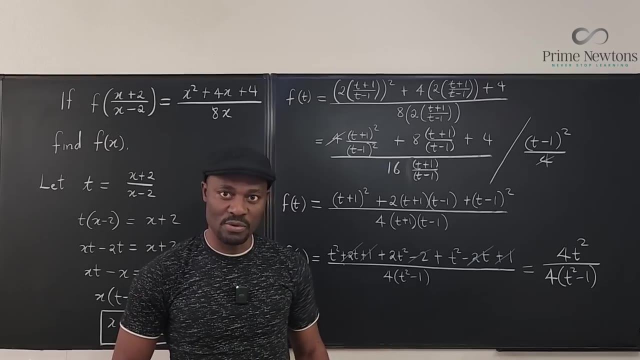 squared, I got four t squared. So this is four t squared over what's in the bottom four into t squared minus one. That's f of t. Now, this is normal. It means I found my answer. Remember the reason we did this substitution is: